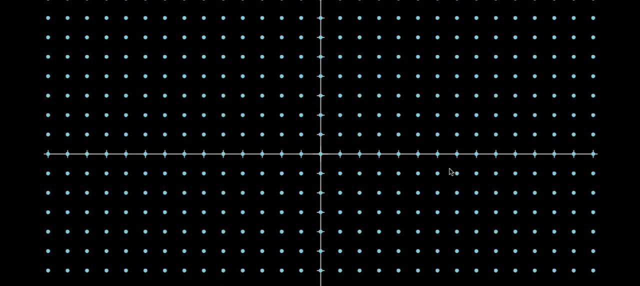 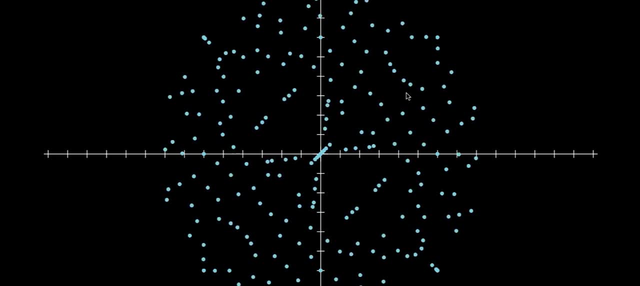 droplets of water And then these are going to start flowing in some way. How would you describe this flow mathematically? So at every given point the particles are moving in some different way Over here they're kind of moving down and to the left. 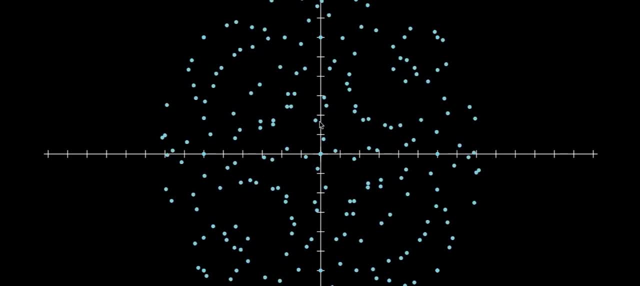 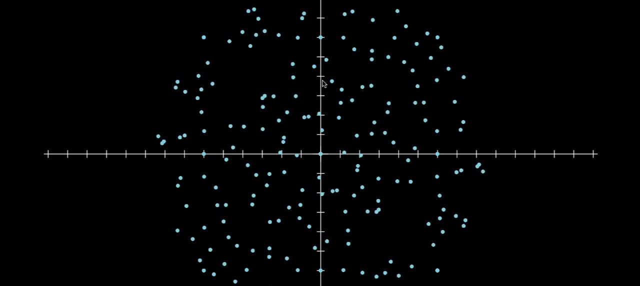 Here they're moving kind of quickly up. Over here they're moving more slowly down. So what you might want to do is assign a vector to every single point in space And a common attribute of the way that fluids flow. this isn't necessarily obvious. 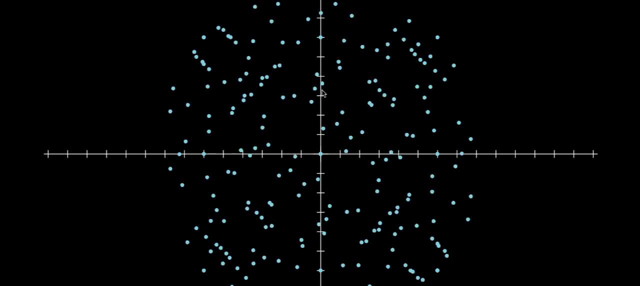 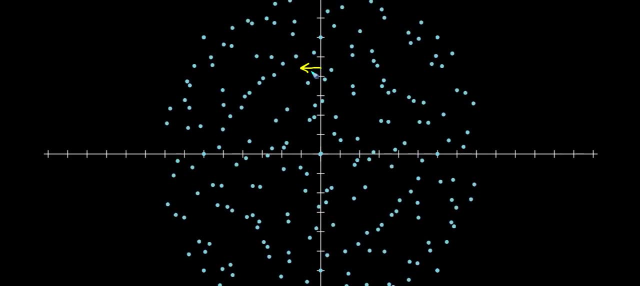 but if you look at a given point in space, let's say like right here, every time that a particle passes through it it's with roughly the same velocity. So you might think over time that velocity would change, And sometimes it does. 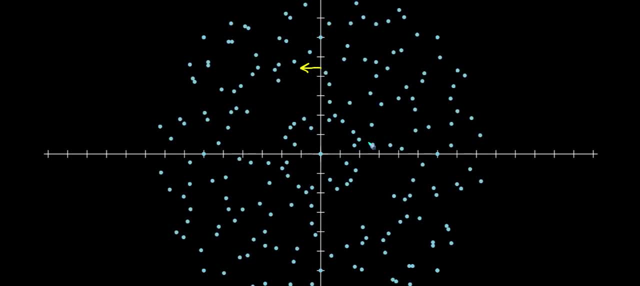 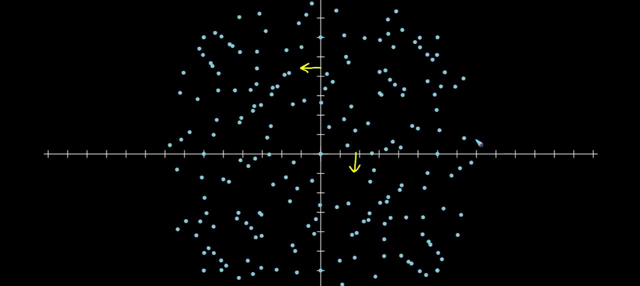 A lot of times there's some fluid flow where it depends on time, But for many cases you can just say: at this point in space, whatever particle is going through it, it'll have this velocity vector. So over here they might be pretty like high upwards. 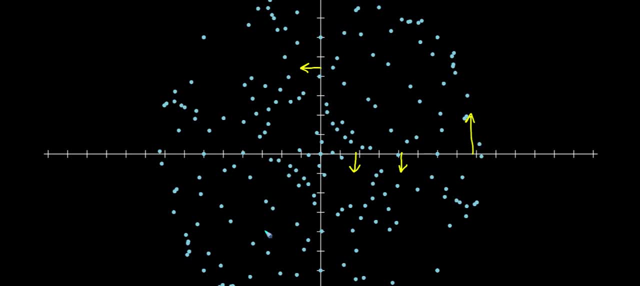 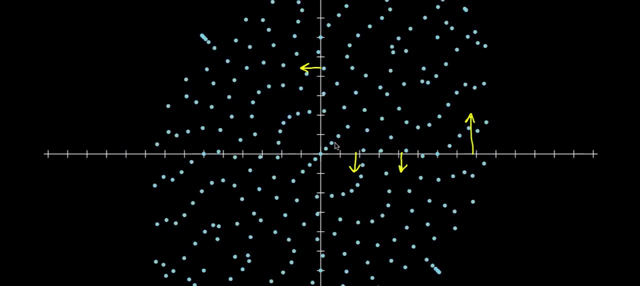 whereas here it's kind of a smaller vector downwards, Even though- and here I'll play the animation a little bit more here- And if you imagine doing this at all of the different points in space and assigning a vector to describe the motion, 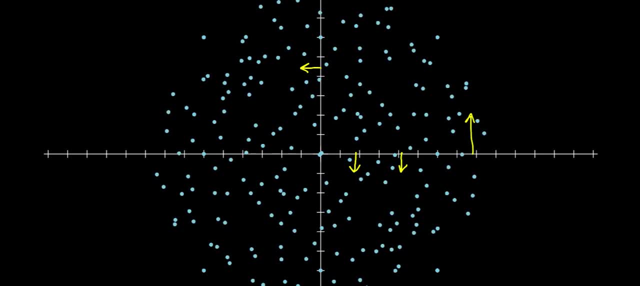 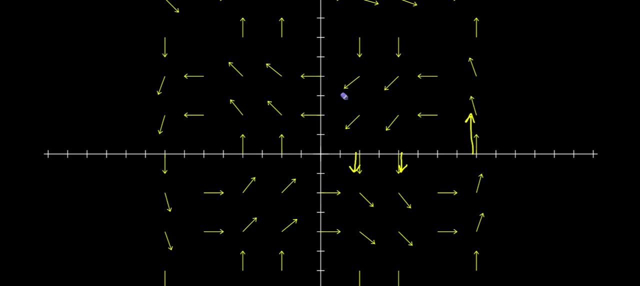 of each fluid particle at each different point. what you end up getting is a vector, A vector field. So this here is a little bit of a cleaner drawing than what I have, And, as I mentioned in the last video, it's common for these vectors not to be drawn to scale. 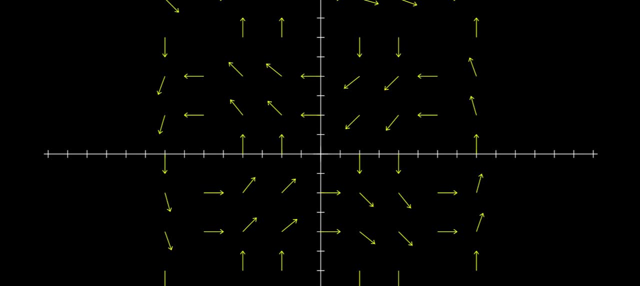 but to all have the same length, just to get a sense of direction. And here you can see each particle is flowing roughly along that vector. So whatever one it's closest to, it's moving in that direction, And this is not just a really good way. 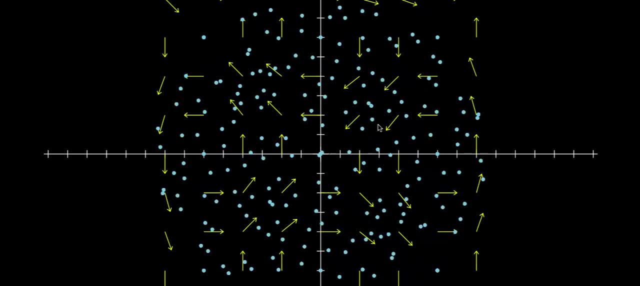 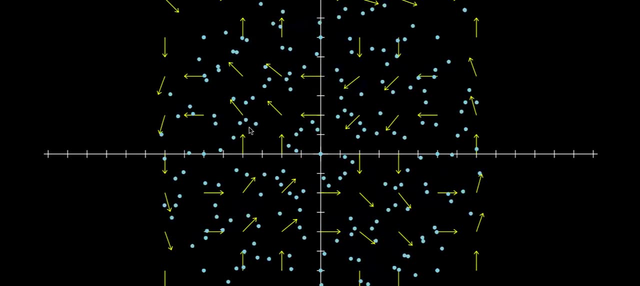 of understanding fluid flow, but it goes the other way around. It's a really good way of understanding vector fields themselves. You might just be given some new vector field and to get a feel for what it's all about, how to interpret it. 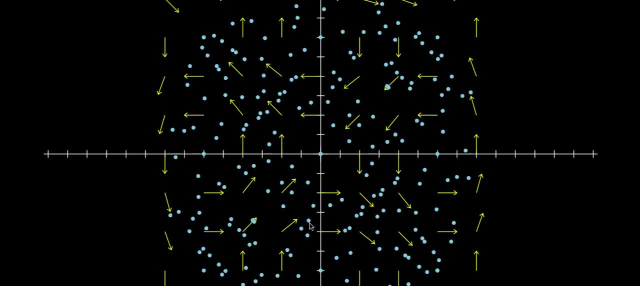 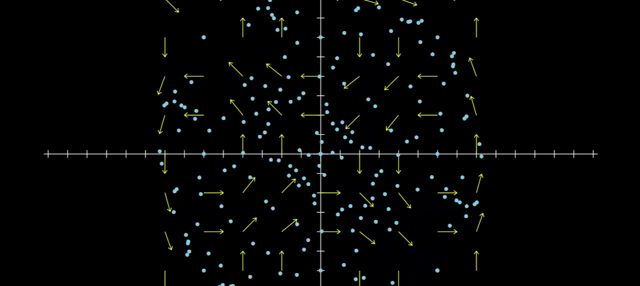 what special properties it might have. it's actually helpful, even if it's not meant to represent a fluid, to imagine that it does and think of all the particles and think of how they would move along it, For example, this particular one. 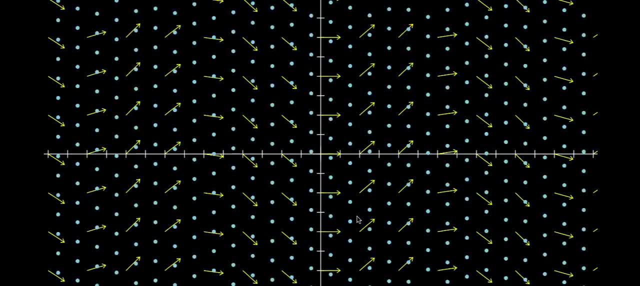 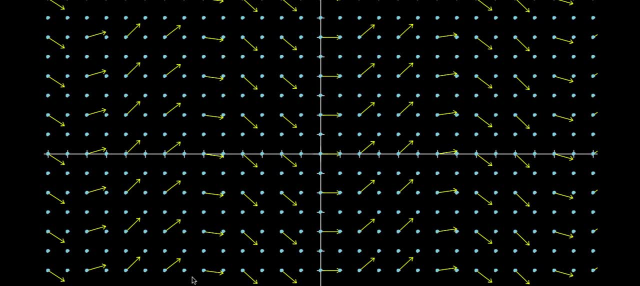 as you play the animation, as you let the particles move along the vectors, there's no change in the density. At no point do a bunch of particles go inward or a bunch of particles go outward. It stays kind of constant. And that turns out to have 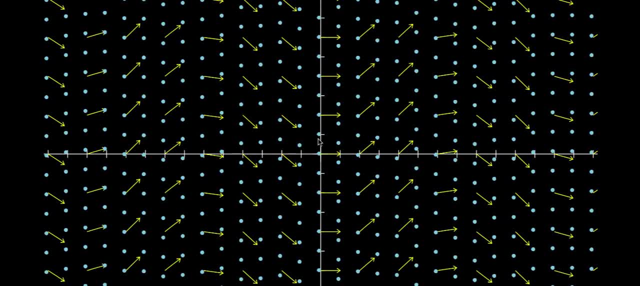 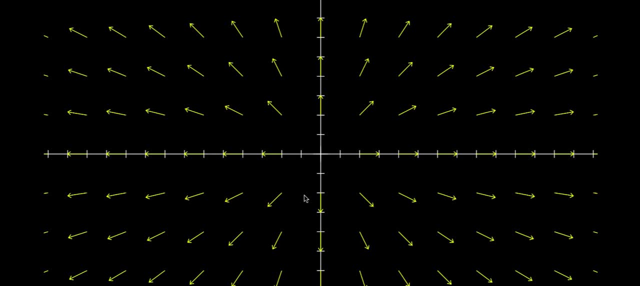 a certain mathematical significance. down the road You'll see this later on as we study a certain concept called divergence, And over here you see this vector field and you might want to understand what it's all about And it's kind of helpful to think of. 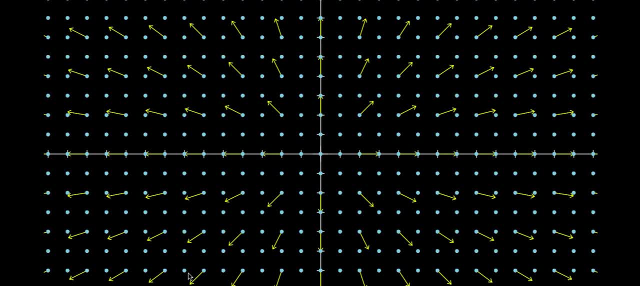 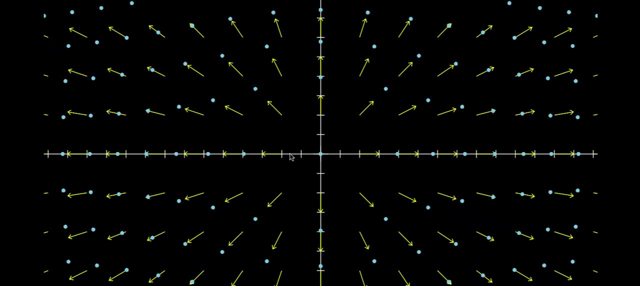 a fluid that pushes outward from everywhere and it's kind of decreasing in density around the center, And that also has a certain mathematical significance And it might also lead you to ask certain other questions, Like if you look at the fluid flow that we started with in this video. 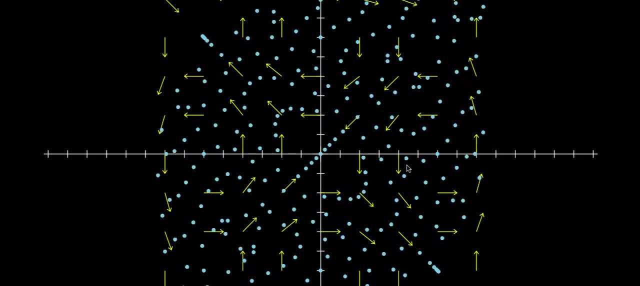 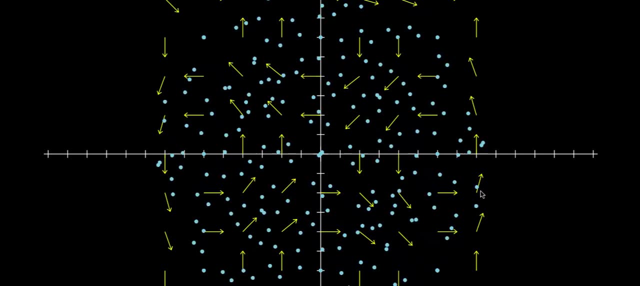 you might ask a couple questions about it. Like it seems to be rotating around some points, in this case counterclockwise, but it's rotating clockwise around others still. Does that have any kind of mathematical significance? Does the fact that there seem to be 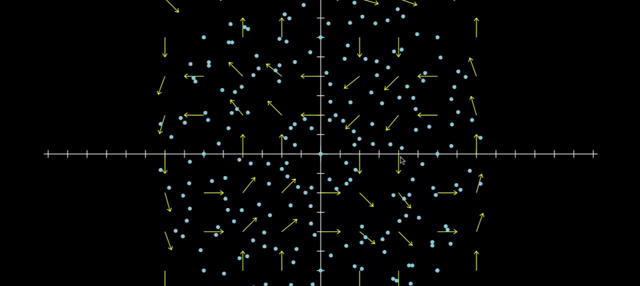 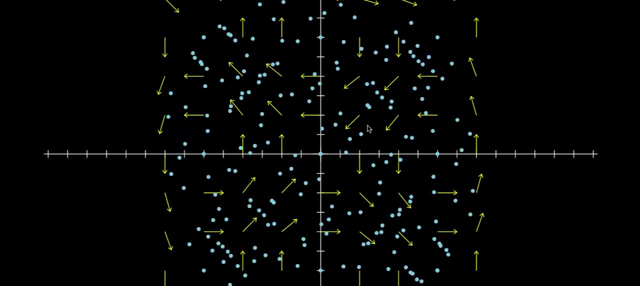 the same number of particles roughly in this area, but they're slowly spilling out there. what does that imply for the function that represents this whole vector field? And you'll see a lot of this later on, especially when I talk about divergence and curl. 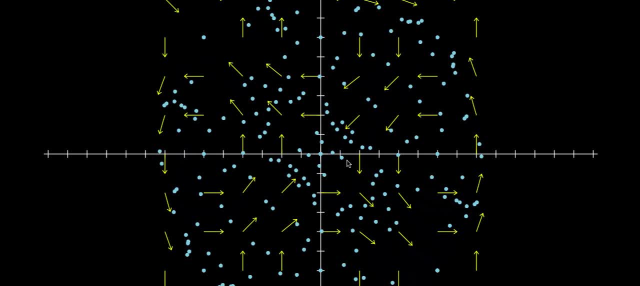 But here I just wanted to show you how to give a little warm-up to that, as we're just visualizing multivariable functions. 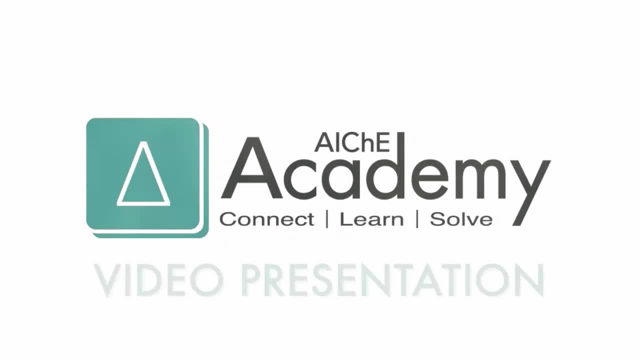 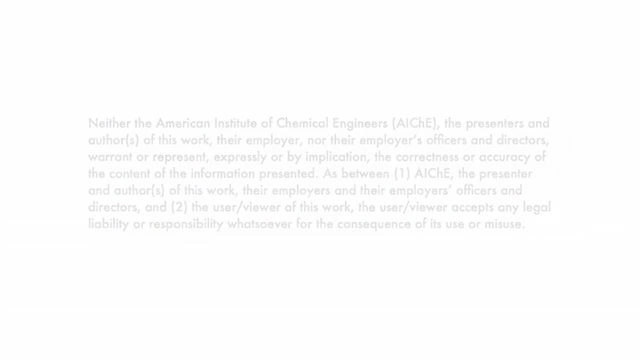 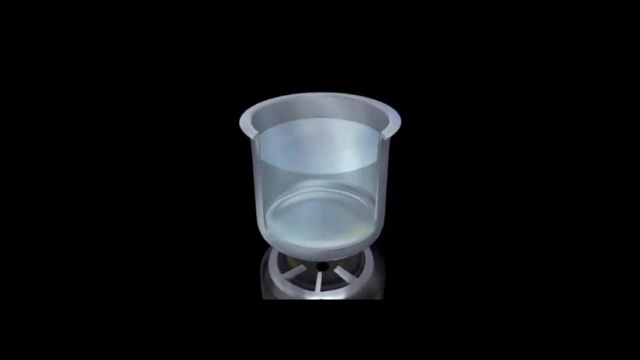 Let's use the example of an ethanol and water mixture. We know that ethanol will boil at a lower temperature than water. Because of this, we say that ethanol is more volatile than water. If we add heat to a 50-50 water-ethanol mixture in a 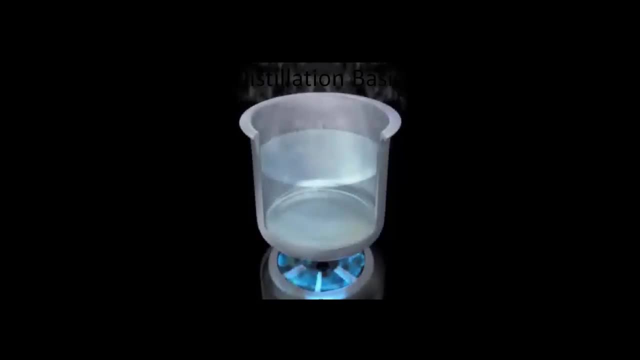 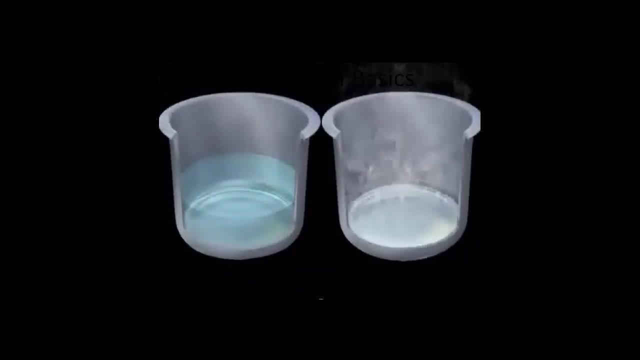 pot. the vapor coming off the top of the pot will be more concentrated in ethanol, since ethanol is more volatile. Likewise, the remaining liquid in the pot will become more concentrated in water. If we collect the vapor from the pot and cool it, it will condense back to a liquid. We end up with two liquid mixtures: one. 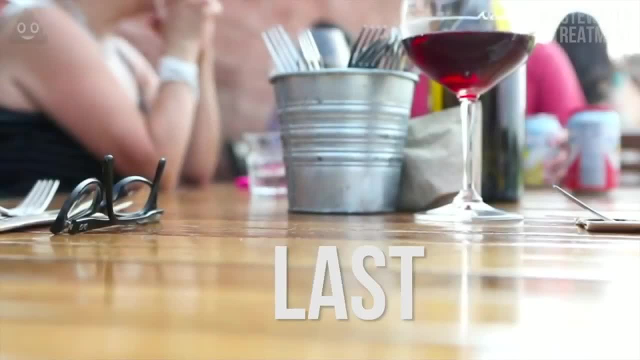 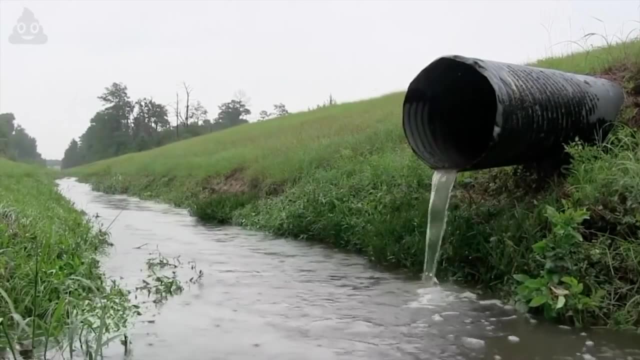 It's a topic we'd rather not think about. Where does last night's dinner go when we flush it down the drain? While you might already be grossed out just thinking about it, this question leads way to a significant subset of civil engineering and a massive amount of public funding, Just like